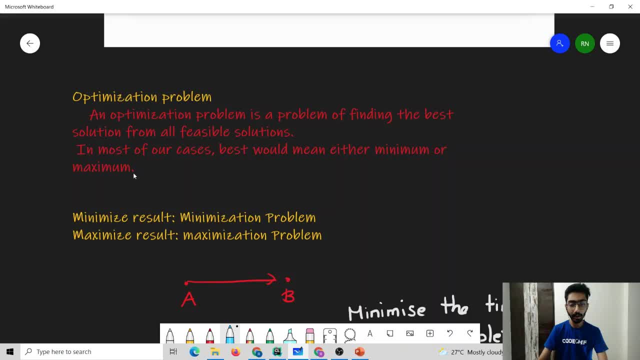 which gives us the minimum result, or something which gives us the maximum result In a problem where we have to minimize some result, we call that problem as a minimization problem, and if we have to maximize a particular result in a problem, we call it as a maximization. 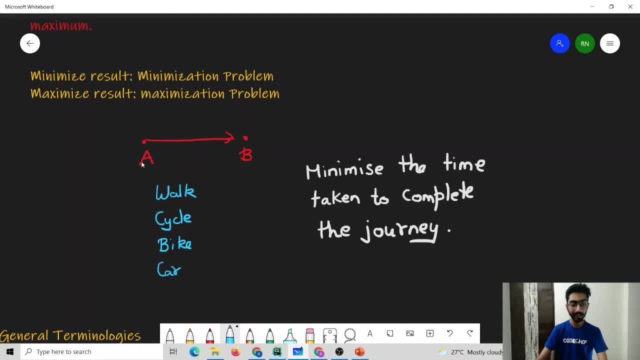 problem. Consider a simple example in which we need to go from point A to point B and we have four options. We can either walk, or we can use a cycle, or we can use a bike, or we can use a car. What we have to do is choose an option such that we minimize the total time taken to complete. 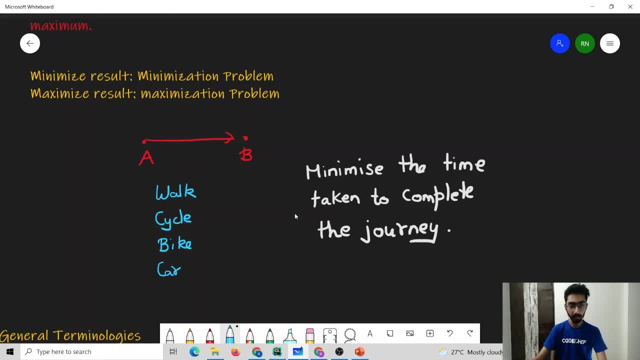 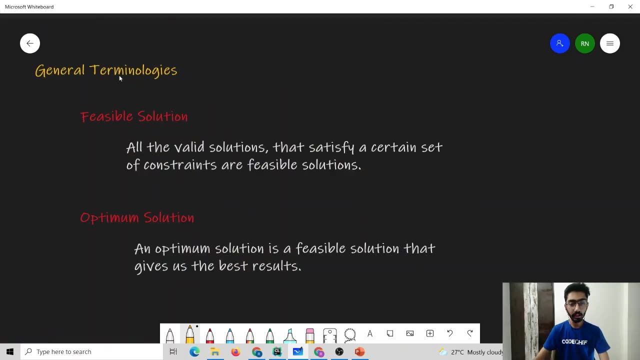 the journey. This is an optimization problem. In particular, this is a minimization problem, because you need to minimize the time taken. For this problem, among these four options, using a car might be the optimum solution. Let us understand a few general terminologies. 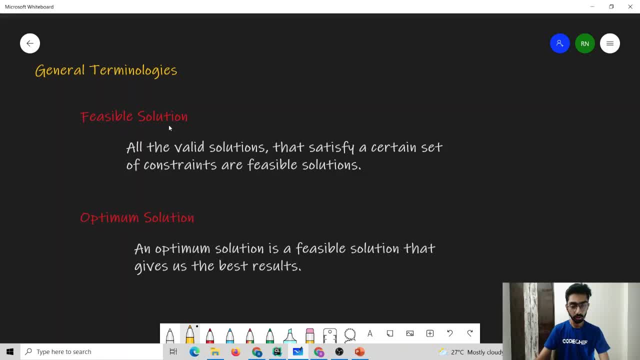 related to greedy algorithms. What is a feasible solution? Feasible solutions are all these valid solutions that satisfy a certain set of constraints. And what is an optimum solution? An optimum solution is a feasible solution such that it gives us the best result, In the example that we have already seen walking or using. 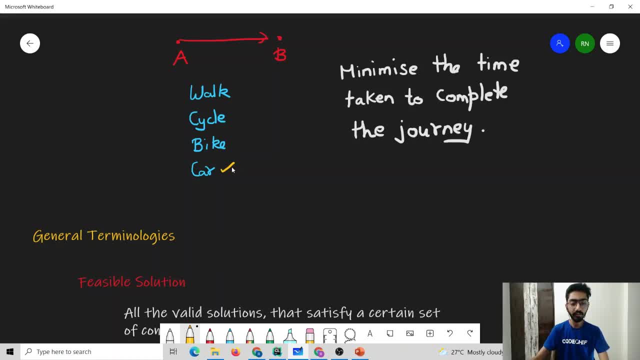 a cycle, or using a bike, or using a car. all these are feasible solutions, But using a car would be our optimum solution. Note that the optimum solution is always a feasible solution. We can not have an optimum solution which is not at all a feasible solution. 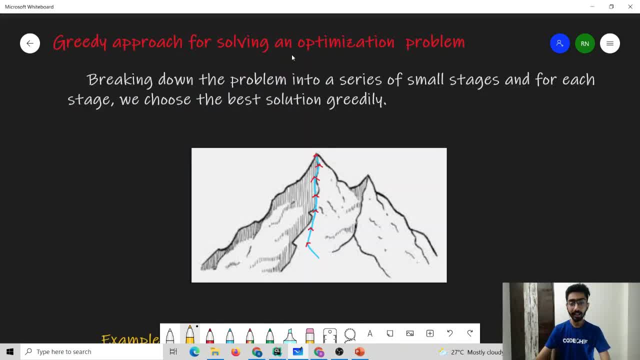 Next we'll try to understand how greedy approaches can be used to solve an optimization problem and what exactly are greedy approaches. So what we can do is there must be one particular problem. We can break it down into series of small stages And for each state we will choose the best possible solution for that. 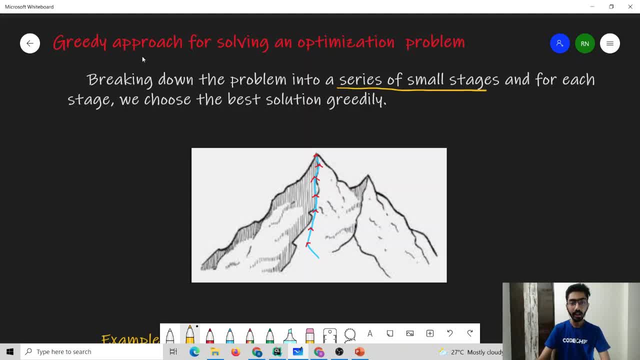 This is how ghillie approaches help us to solve a particular problem, like for this example. if we want to move from this point to this point, at every step we will look for the direction which gives us the steepest increase in height. after that we will take that move then again. 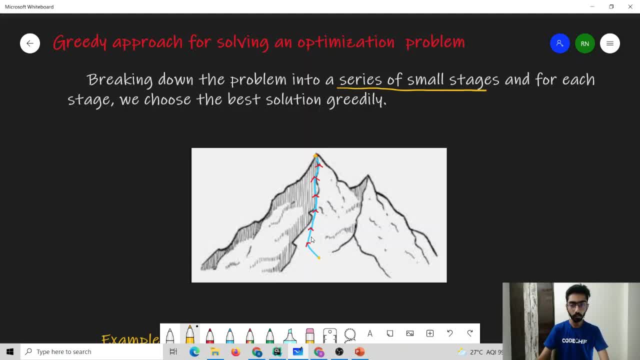 we will look for the steepest increase in height and we will take that move slowly, slowly, we will take our ghillie moves and finally we will reach our optimum solution, which is the peak. so what ghillie algorithm does is every time it will look at a very small sub. 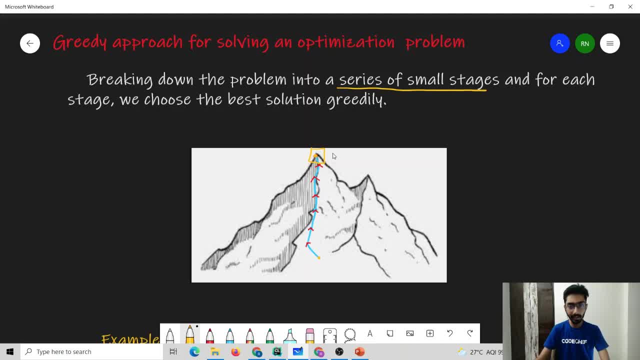 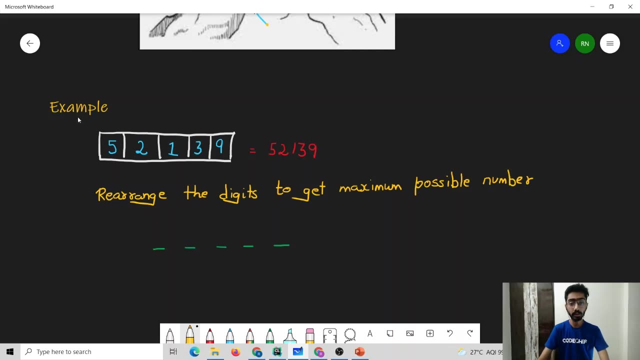 problem or a very small stage, and it will try to solve this small stage, ghillie and by taking such small, small ghillie steps. finally, we are going to get to our optimum solution. a simple example for a problem which can be solved by using ghillie approaches: consider: 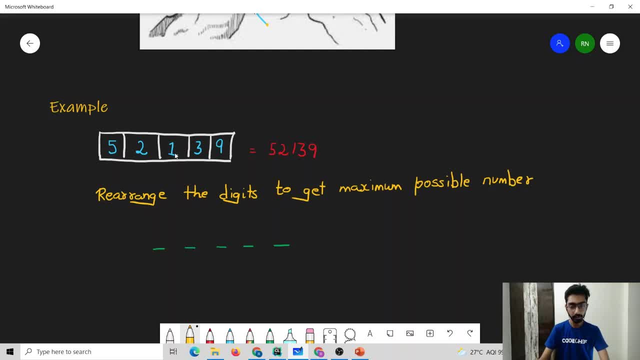 that you have been given an array which consists of some number of elements, and now you want to rearrange the digits in this array such that you can maximize the possible number. and what's the possible number? it's the number that is formed by just concatenating all the 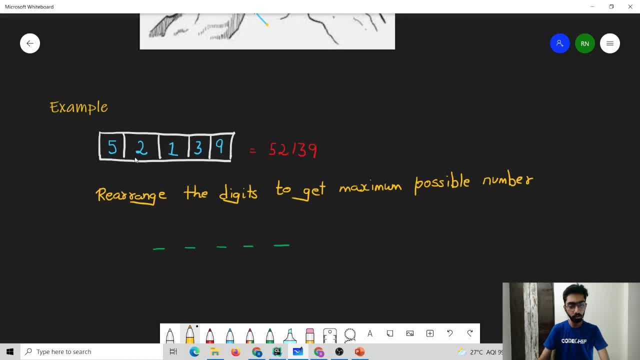 digits in the given order, like, if the array is 5, 2, 1, 3, 9, then the number we are going to consider is going to be 5, 2, 1, 3, 9, which is 52139. so what we have to do is we have. 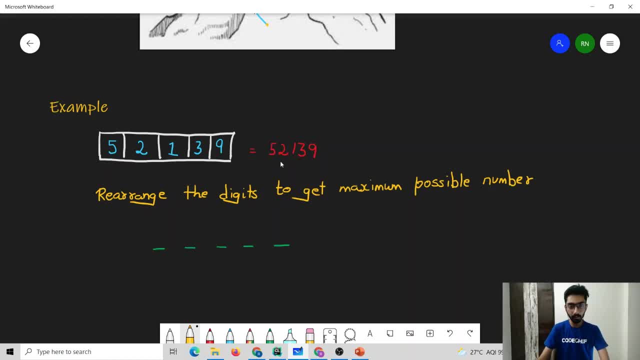 to rearrange the elements in this array such that the number that will be formed is maximized. what ghillie approach can we use? what we can do is, at every step, we can try to fill only one element, which is the element which is at the highest position. and what we can 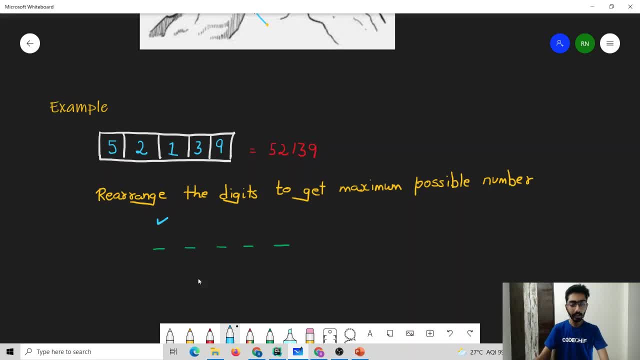 do is we can try to fill this position by the largest possible number. for example, when we are trying to fill this particular position, we have to find the largest possible number in this array. the largest possible number is going to be 9, after which we remove 9 from. 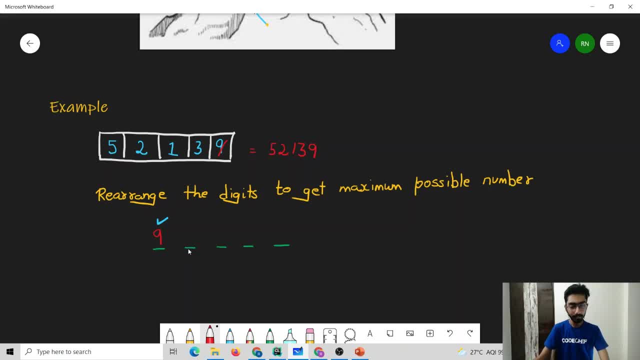 our array. So if we look again, ghillie, which is the largest position, it will be 5. then again we will remove 5, and then we have ghillie wheelchair, which is the largest number left. again it will be 3, then ghillie wheelchair, which is the largest number left, which will be 2, and then 1 in. 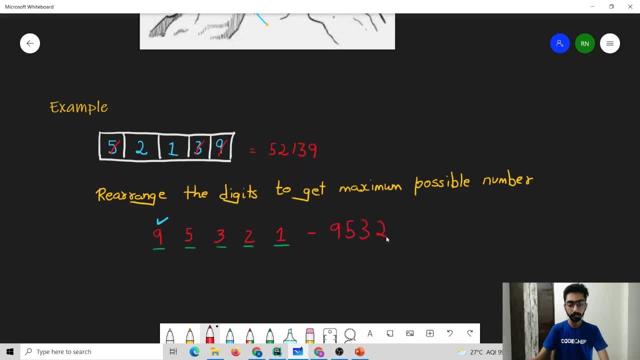 this way we will get 95321. so what we have done: in every step we have, ghillie, chosen the best possible value for that step And in that way we are hoping that the final result that we get is the best possible value, and in this case it is indeed the best possible value. 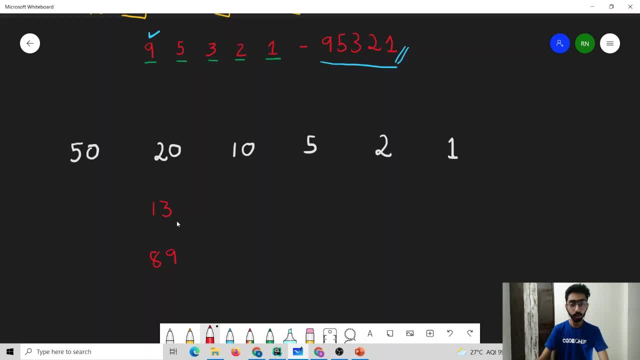 Knowingly or unknowingly, we all have been using ghillie algorithms throughout our life. Consider a simple day to day life problem. consider you have many currency denominations of all these kind of nodes, that is, 50 rupees, 20 rupees, 10 rupees, 5 rupees and 2 rupees. 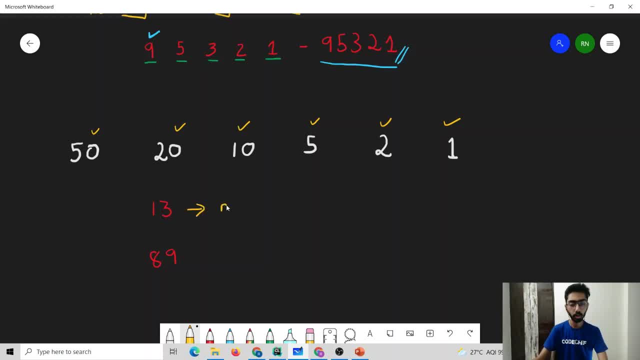 and 1 rupee. And what you need to do? What you need to do is we have to use the minimum number of nodes that is possible. Isn't this a problem that we have been solving throughout our life? So how can we use the minimum number of nodes? 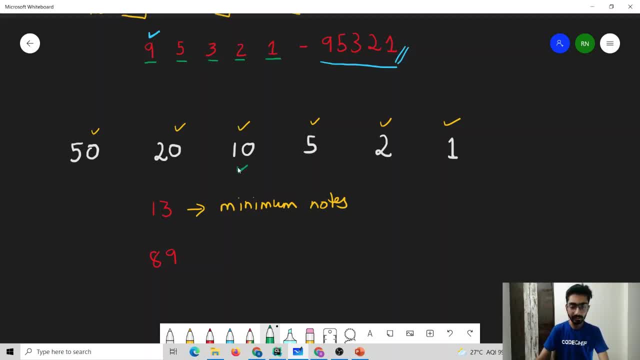 What we generally do is we try to find the highest node that can be possibly used by us. in this case, for 13 rupees we can at max use a 10 rupee node. So we will use a 10 rupee node. then we will be left with 3 rupees. then we will again check. 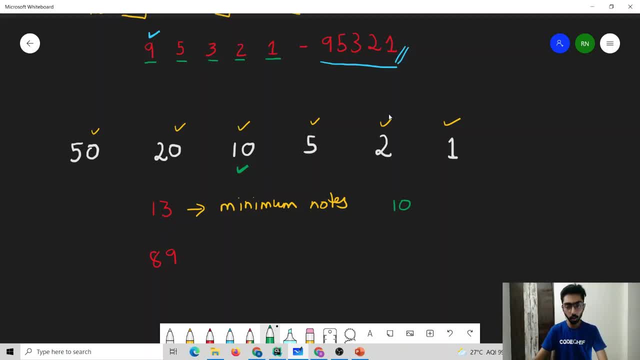 which is the largest node that can be used. We will get to know that only 2 rupee node can be used, So we will then use a 2 rupee node and then we will be left with only 1 rupee, and then 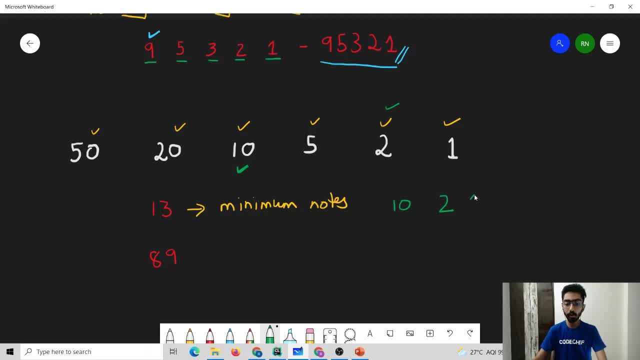 we will check and find that only 1 rupee node could be used. So we will use a 1 rupee. So indirectly, we are just using 3 nodes to get a sum of 13 rupees. Similarly, if we need to find the number of nodes required for 89 rupees, we will first 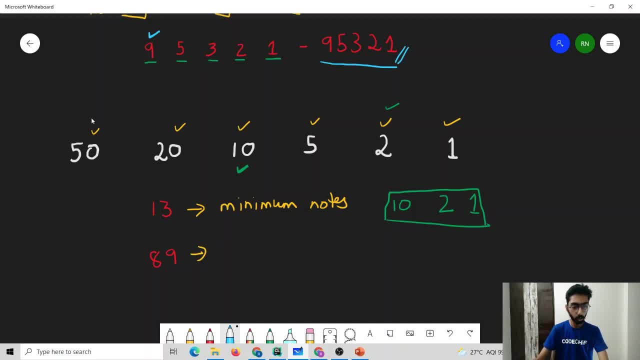 check which is the largest value that can be used, we get to know that it is 50. So we will use a 50 rupee node, After which we again check which is the largest value that can be used. we are left with only 39 rupees to form, and we get to know that 20 rupee can be used. 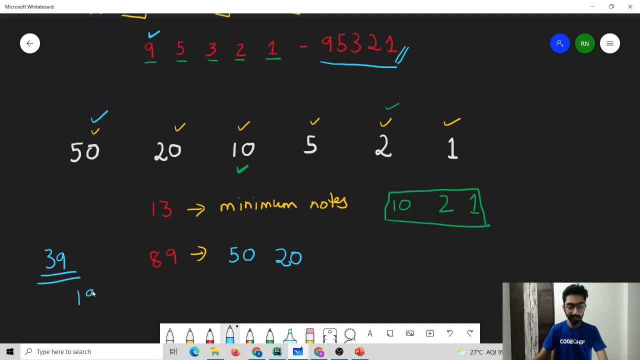 So we will use a 20 rupee node. Then we will be left with 19 rupees and we will use a 10 rupee node, After which we will be left with 9 rupees, and for 9 rupees, what we will do? we will use